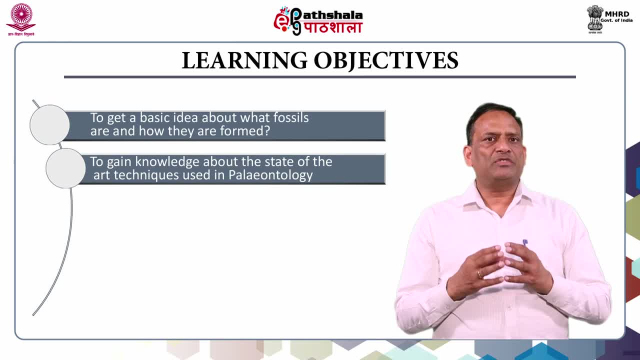 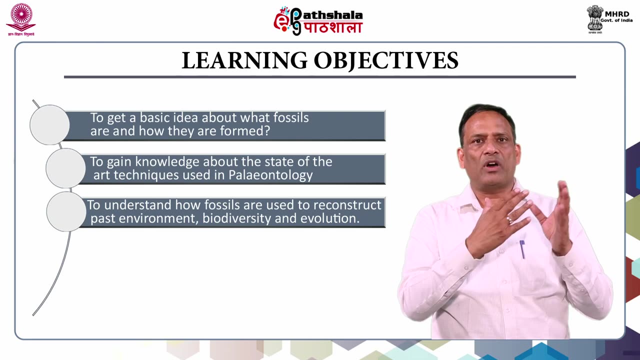 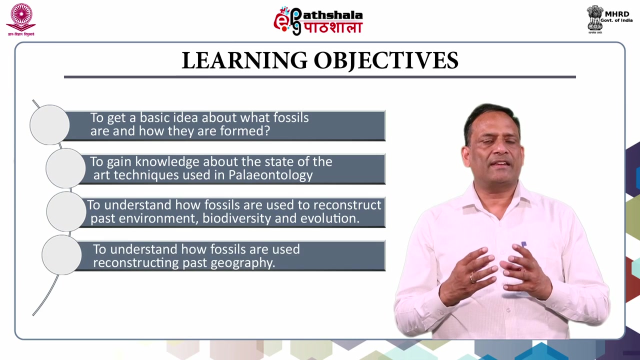 are and how they are formed. Second objective of this module is to gain knowledge about the state of the art techniques used in paleontology. The another objective of this module is to understand how fossils are used to reconstruct past environment, biodiversity and its evolution. And the last objective of this module will be to understand that. 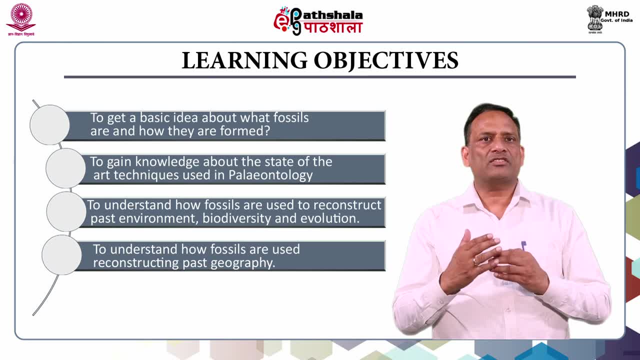 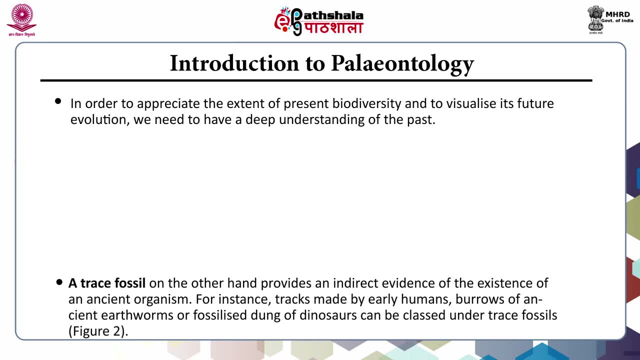 how fossils are used, reconstructing past geography. In order to appreciate the extent of present biodiversity and to visualize its future evolution, we need to have a deep understanding of the past. Paleontology is one such science that provides us a window into the past life. 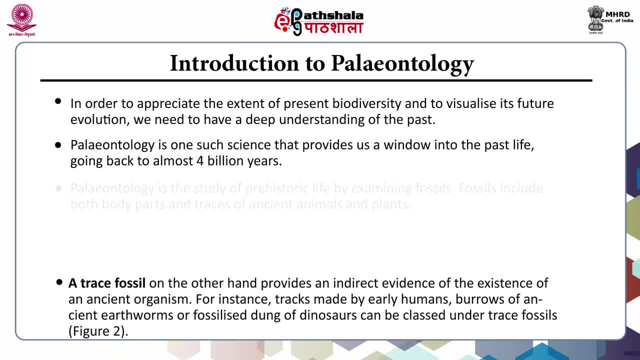 going back to the almost 4 billion years. In the first module, you have learned about paleontology. In the first module, you have learned about paleontology. In the first module, you have learned about geological time scale and that is very important here in paleontology arts. 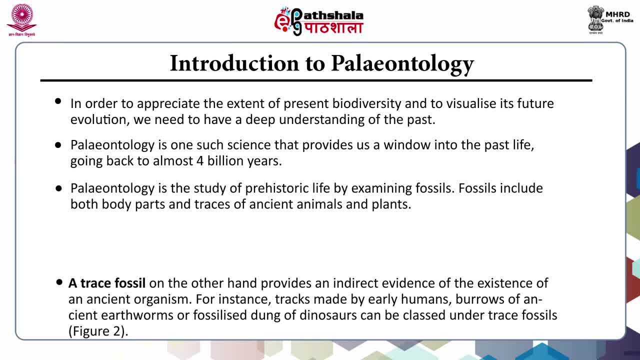 To introduce the subject of paleontology. paleontology is the study of prehistoric life by examining the fossils. These fossils include both body parts and traces of the ancient animals and plants. So we can say that fossils are of two types: body parts and the traces. 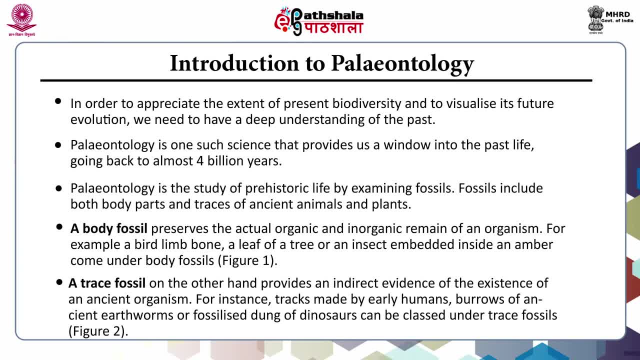 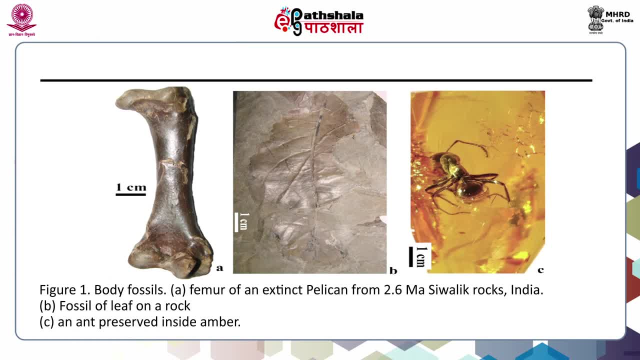 Now, a body fossil preserves the actual organic and inorganic remain of an organism. Let me take an example: that a bird's limb bone that can be a fossil or that will come under the category of body fossil. Similarly, a leaf of a tree or an insect embedded inside an umber come under body fossil, A trace fossil. 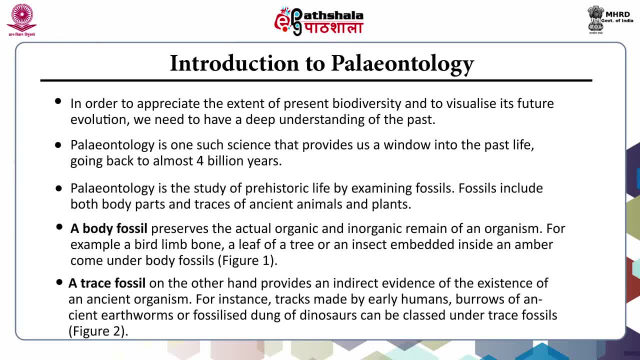 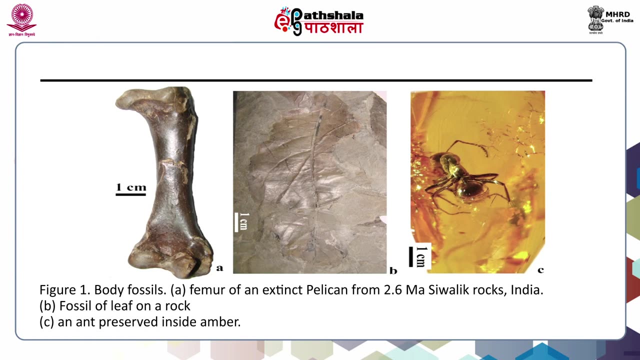 on the other hand, provides an indirect evidence of the existence of an ancient organism. For instance, tracks made by early humans, burrows of ancient earthworms or fossilized dung of dinosaurs can be classed under trace fossils. Let me show you a figure In this figure. 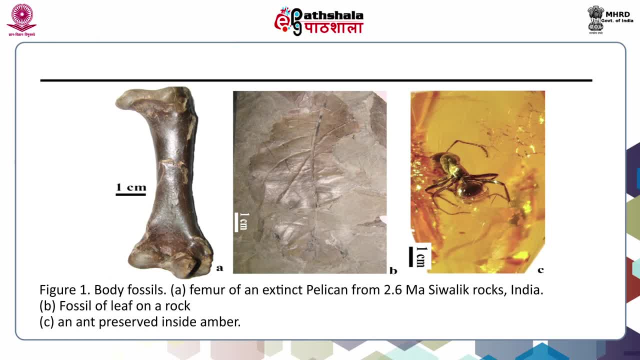 there are three pictures of the fossils. The first picture is of a femur, of an extinct pelican, from two points, five, six million years ago, from Shivalik Rocks, India. Second fossil that is in between, in between the three, that fossil of leaf on a rock. and third one is a fossil of an ant. 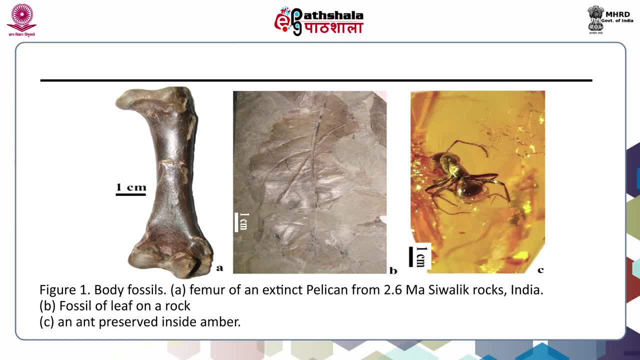 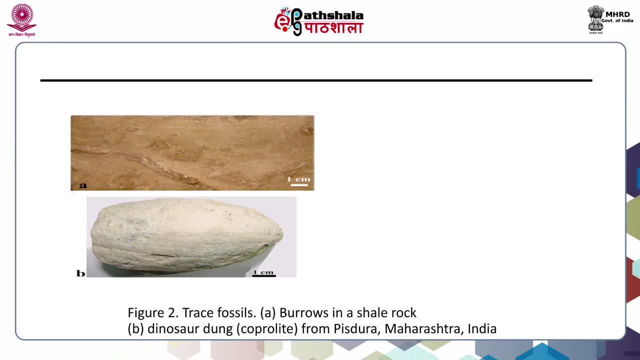 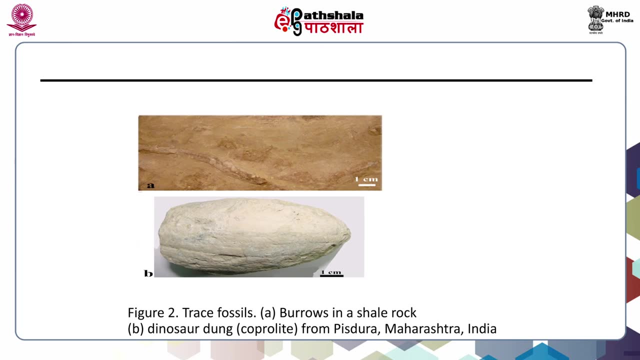 that is preserved inside the umber. So these all, the three- are examples of body part fossils. Now let me have a look on this. these two pictures. These are the examples of trace fossils. First one is the example of a burrow that is in a shale rock and second one is the 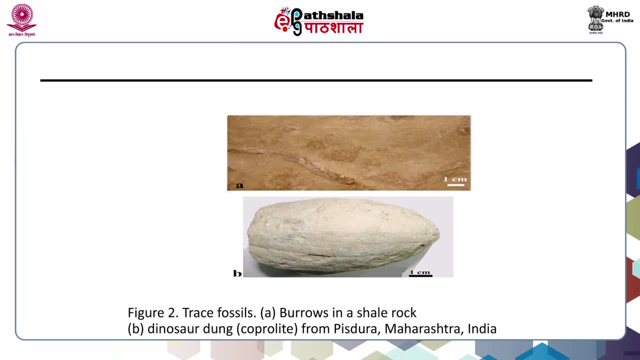 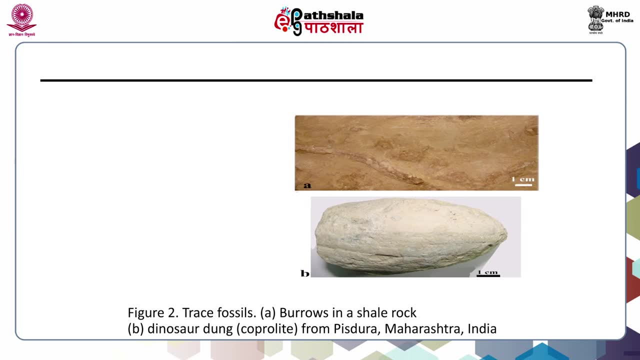 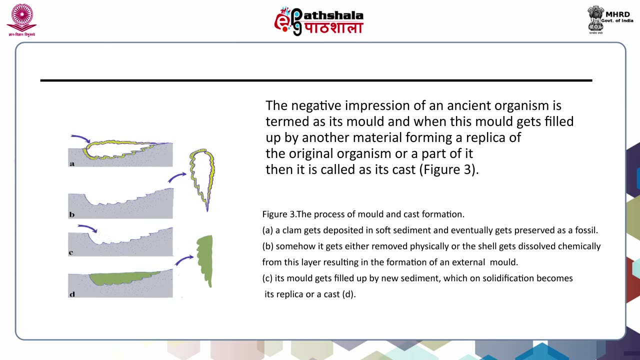 example of a dinosaur dung. This dinosaur dung, these dung fossils, also called as coprolite, and these pictures are from Pisdura, Maharashtra, India. Let me have a look on this slide. The negative impression of an ancient organism is termed as its mould. 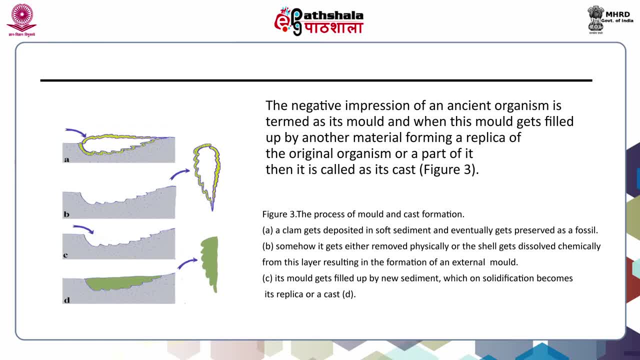 And when this mould get filled up by another material forming a replica of the original organism or a part of it, then it is called as its cast Means. there may be mould and cast. Let me have a look on these pictures. The process of mould and cast formation is shown in these. 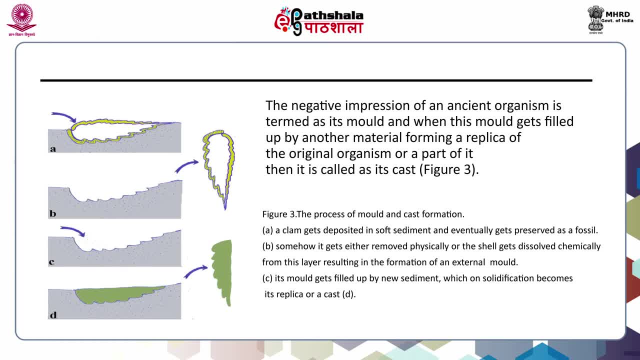 diagrams. The A figure is showing a clam. Clams are nothing, but these are bivalve mollusks. So a clam gets deposited in soft sediment and eventually get preserved as a fossil. That is shown in the picture A. Now look at the picture B. Somehow, due to one or other reason, this clam that was deposited 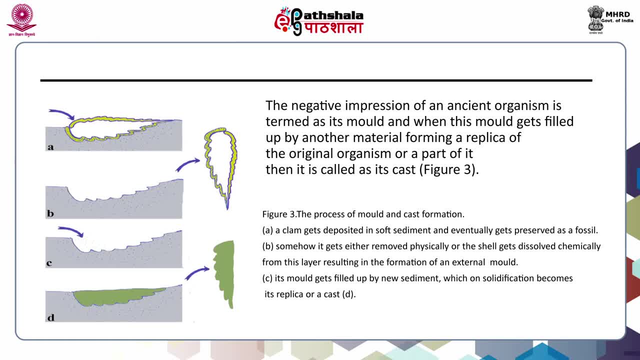 over there that gets either removed physically or by the shell, gets dissolved chemically from this layer throat, remove cities in the dirt relief And this result in the fossil melt chocolate Localization is going on and nature pegar formation of an external mould and the mould that will be formed that is shown in the figure. 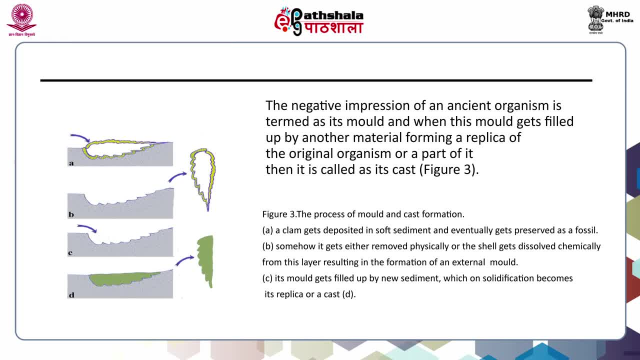 B. Then this mould get filled up by new sediment which on solidification become its replica. This is shown in filling of this mould is shown in the figure C, and then forming of the cast is shown in the figure 4.. So we can get this type of fossils also, which are: 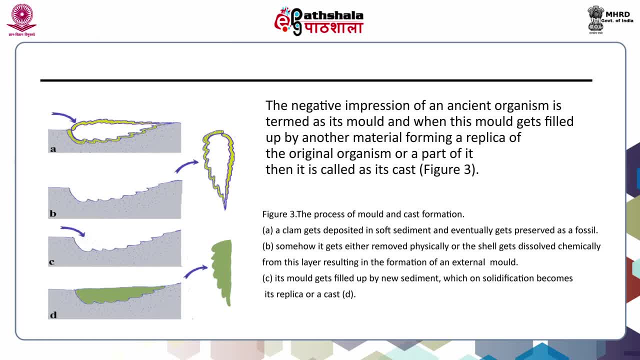 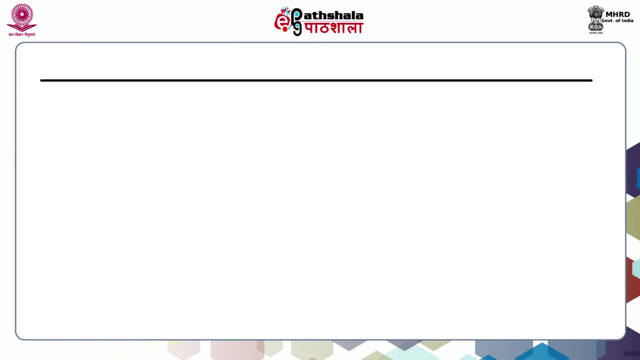 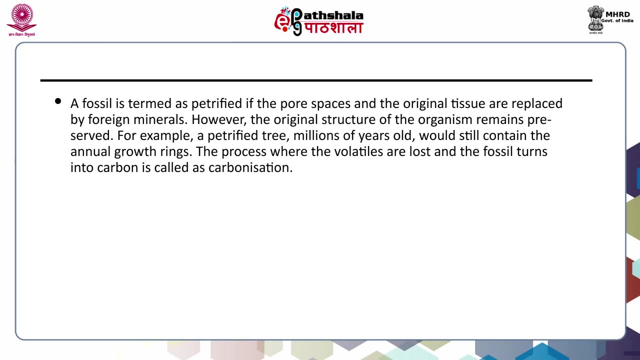 produced by some other material, from the moulds of, from the moulds prepared by different organisms in the past. Now, what is a fossil Fossil is termed as petrified if the pore spaces and the original tissue are replaced by foreign minerals. 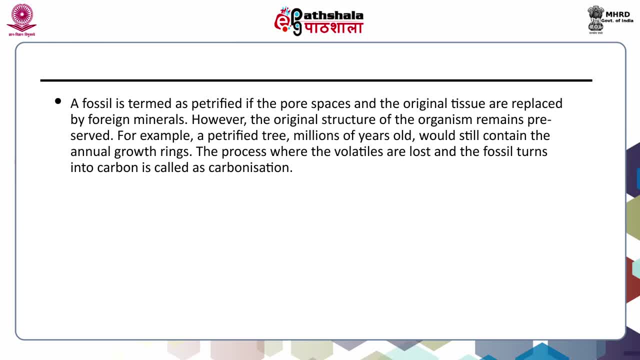 However, the original structure of the organism remains preserved. For example, a petrified tree, millions of years old, would still contain the annual growth rings. The process where the volatiles are lost and the fossil turns into carbon is called as carbonization. 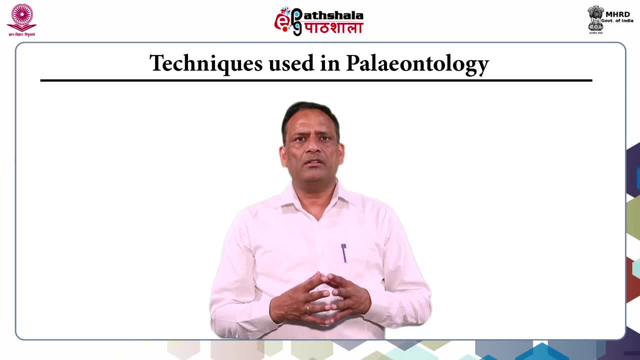 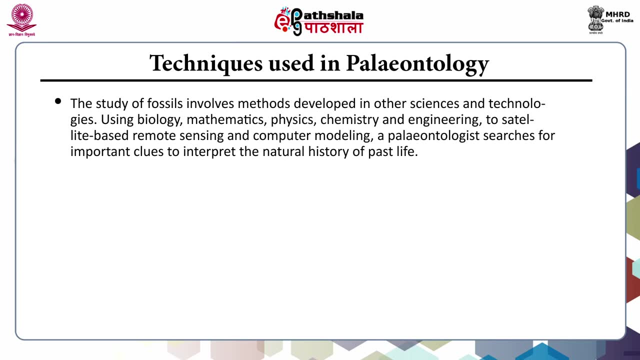 Several techniques are used in the paleontology. A student of paleontology must have the knowledge of the paleontology, So the study of fossils involves methods developed in other sciences and technologies using biology, mathematics, physics, chemistry and engineering to satellite based remote. 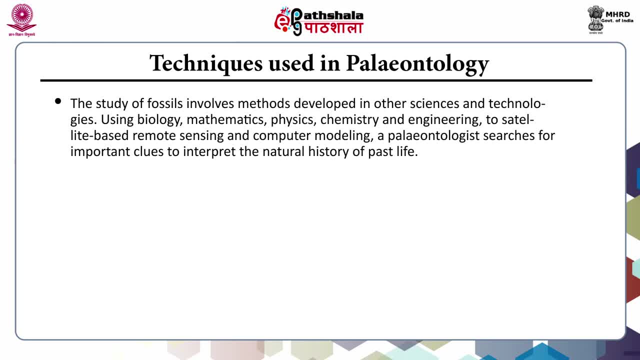 sensing and computer modeling. A paleontologist searches for important clues to interpret the natural history of past life. So we can say that a geologist should have the basic knowledge of all the sciences, including biology, mathematics, physics, chemistry, engineering. 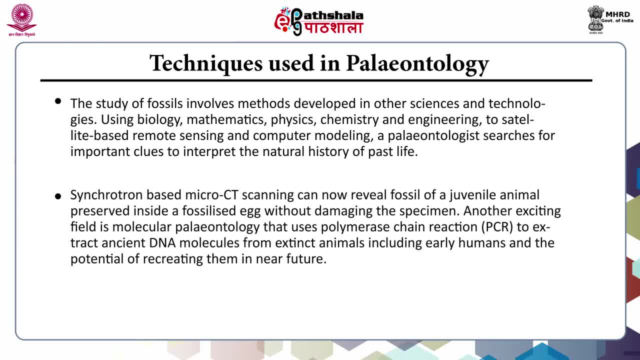 remote sensing, etc. etc. A synchrotron-based micro-city scan can now reveal fossils of a juvenile animal preserved inside a fossilized egg without damaging the specimens. Means what I want to say: that nowadays such type of technologies are available to us, which 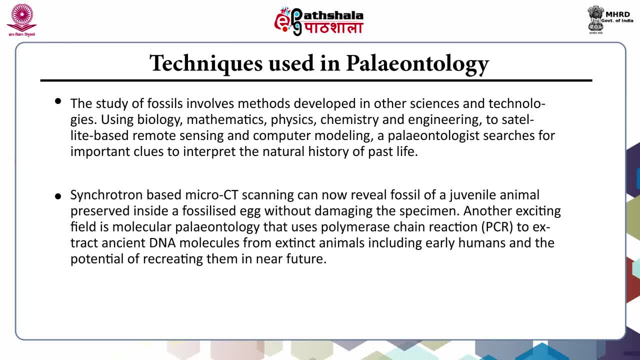 can be used To reveal the information from the fossil without doing any kind of damage to the specimen. Other exciting field is molecular paleontology that uses polymerase chain reaction. Polymerase chain reaction is a very common technique for the biologists, So this technique can. 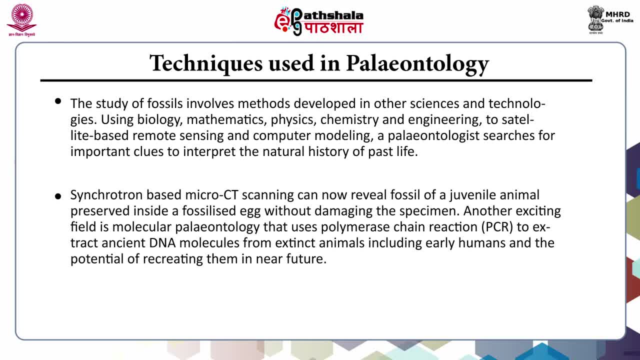 be used here in the paleontology also. Basically, this technique is used to extract ancient DNA molecules from exoskeletons. So this technique can be used to extract the DNA molecules from extinct animals, including early humans, and the potential of recreating them in near future. More importantly, paleontology. 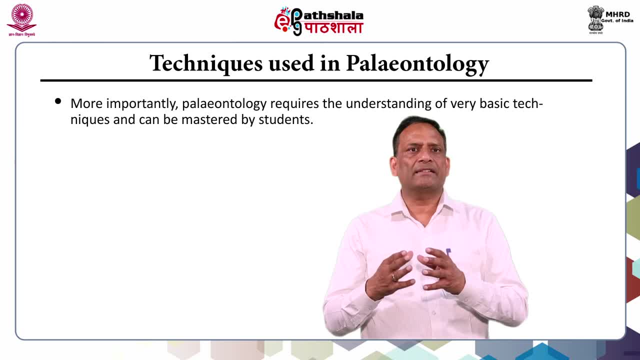 requires the understanding of very basic techniques and can be mastered by the students. Fossils are first discovered in the field where natural erosion or excavation exposes fossil bearing rocks. Fragile rock, Fragile fossils require extreme care and often are glued with the matrix to avoid damage. 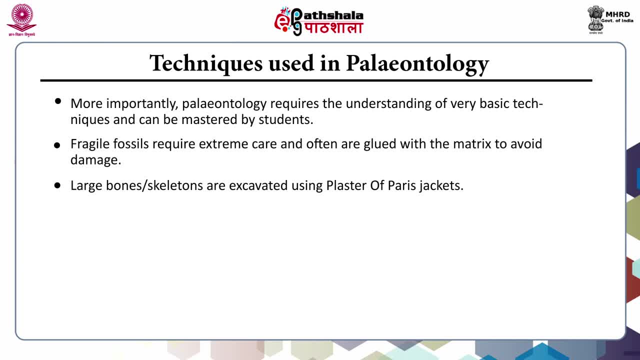 Large bones and skeletons are excavated using plaster of Paris jackets. A field paleontologist is required to take photographs by placing a scale close to the fossil before removing it. So camera, So camera. The photographic camera is very, very important for any paleontologist. and we place this scale. 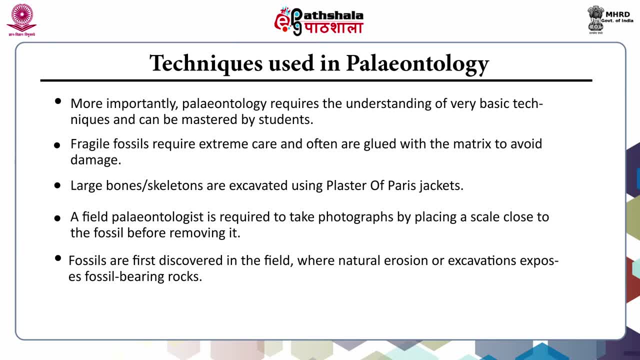 close to the fossil. that will give us an idea of the size of the fossil. Collected fossils are catalogued in the field diary and information about the precise geographic location using a GPS is noted. This noting of geographical location using GPS is highly important, So 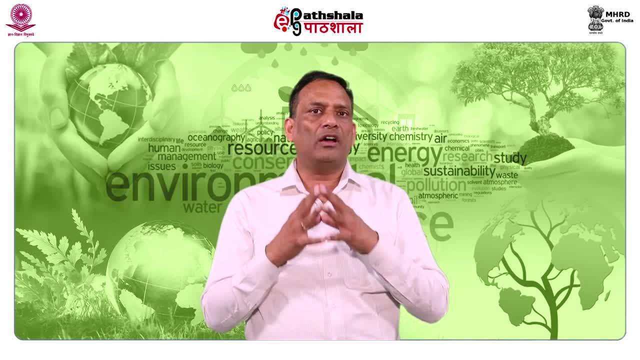 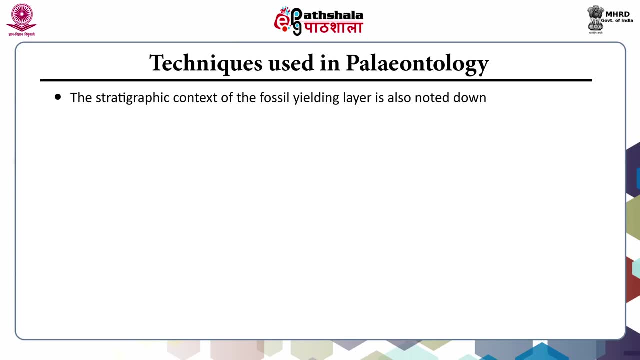 this is a very important technique. The photographic camera and information using GPS is also another important component of field studies. in the field of geology, The stratigraphic context of the fossil in the yielding layer is also noted down. For micro fossils, bulk samples are collected from specified 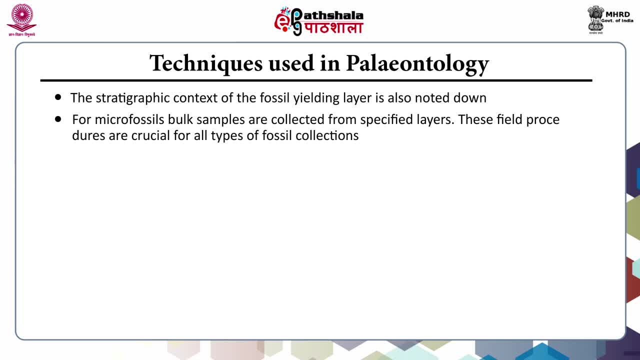 layers. These field procedures are crucial for all type of fossil collections In the laboratory. the fossil concepts are taken from the data collected by the laboratory, are cleaned and restored. if damaged, If fragmented or disarticulated, they are rejoined and reconstructed as close as possible to their original state. Micro fossils are recovered from sediments. 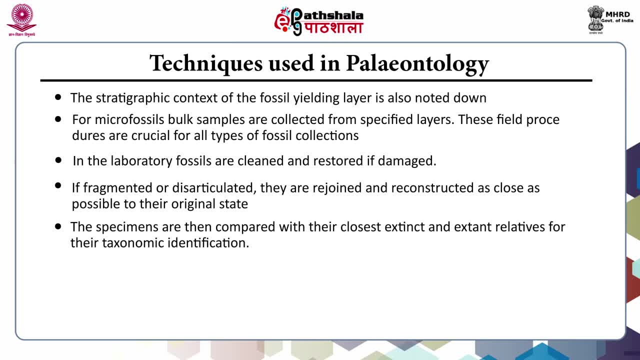 by soaking them in water or other solvents and screening through sieves. The specimens are then compared with their closest extinct and extent relative for their taxonomic identification. Fossils are then numbered and catalogued in a book or a or on a computer. Replicas of 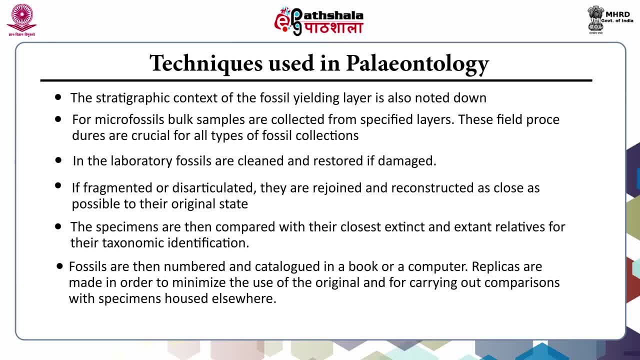 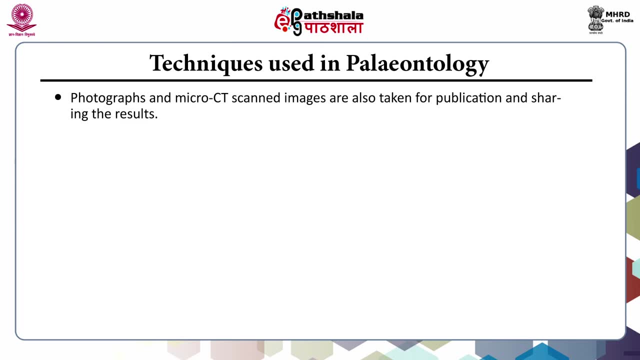 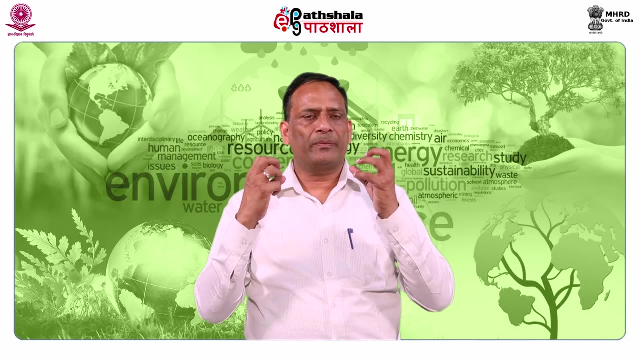 these fossils are made in order to minimize the use of the original and for carrying out comparisons with specimens. How about elsewhere? Photographs and micro city scanned images are also taken for publication and sharing the results. So the student must know that how the replicas of these fossils 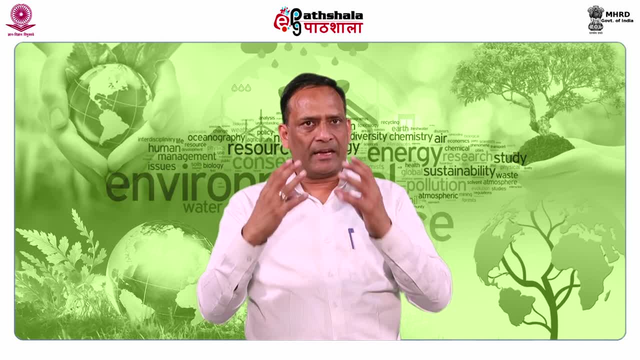 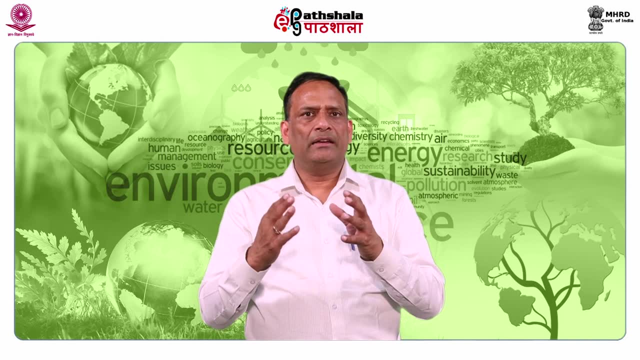 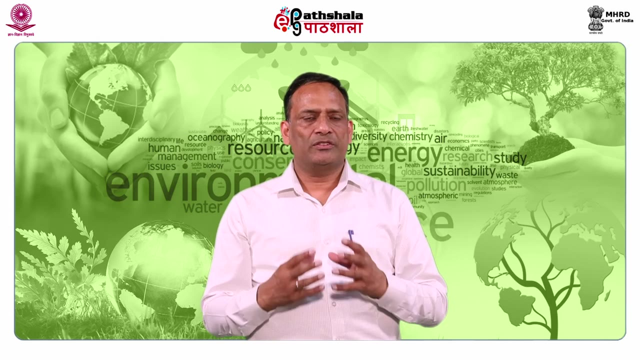 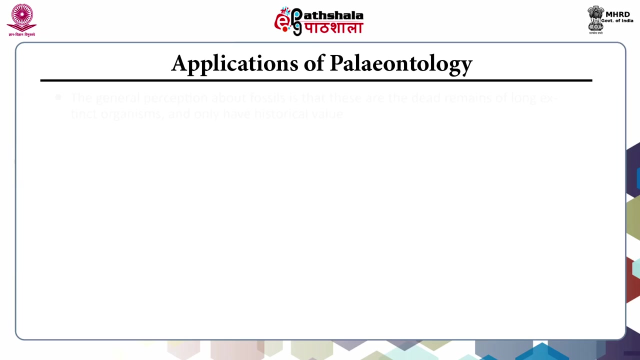 are formed. Preparation of for these replicas is very, very important because by making the replicas, we can avoid the time and again handling and dealing of the originals. Now the question arises: What are the replicas from the images that were found? What are the applications? 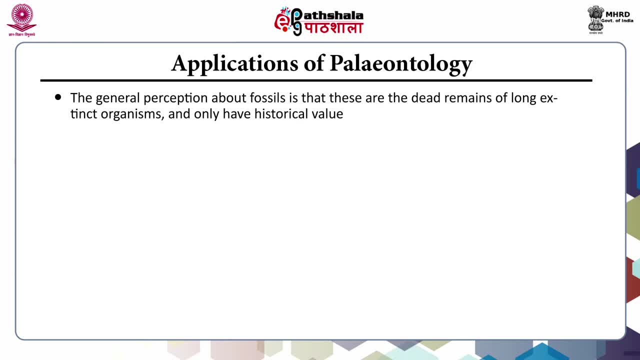 of paleontology. Paleontology is having lot of applications in almost every field of the science. Otherwise, the general perception about fossils is that these are the dead remains of long extinct organism and only have historical value. but this is not the case. Lot of information. 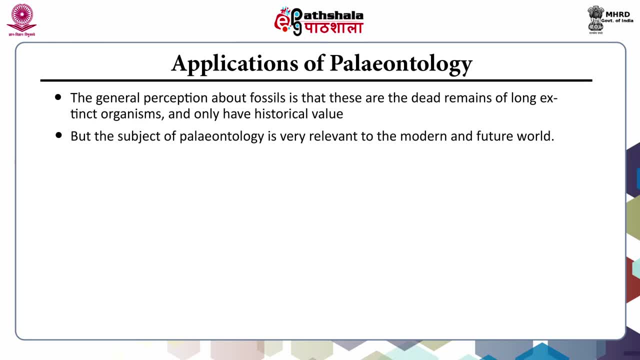 can be drawn from the fossils. paleontology is very relevant to the modern and future world. By paleontology we get to know how, when and why the early organisms developed, how land masses have moved across the globe and how climate has changed over the years. and 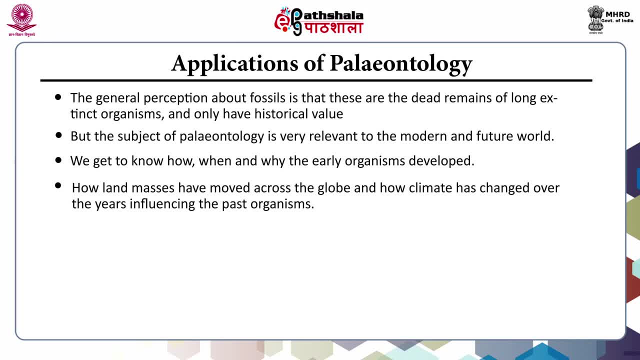 how it has influenced the past organism, how past organisms have changed the physical features of this worlds. So this, all information can be derived from the fossils. Fossils tell us about extinctions, evolutionary changes and changes in the biodiversity over the past several million years. 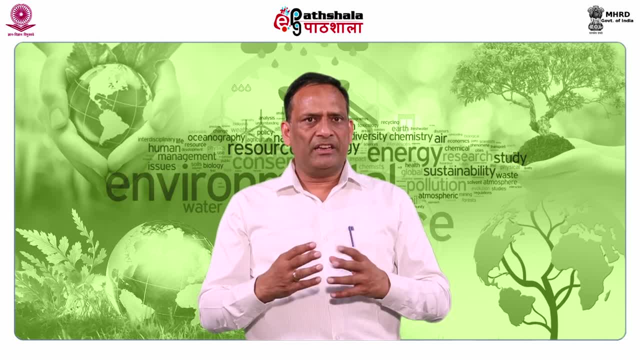 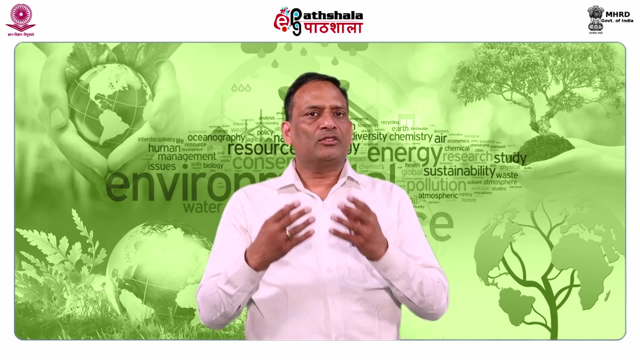 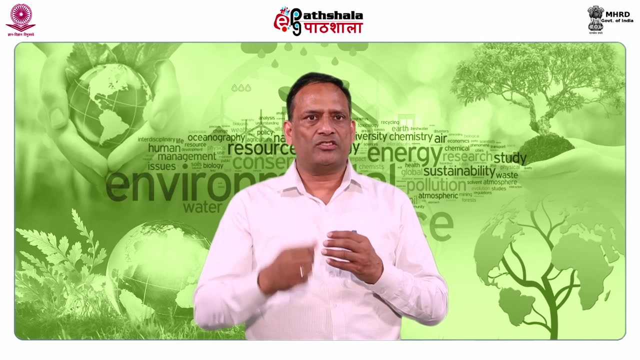 The study of paleontology has got several applications. Let me take one example. Fossils can be of economic importance also, as well as of academic value, Since petroleum and coal are basically the product of ancient organisms. so the study of fossils is imperative for oil and coal exploration as well as exploitation. 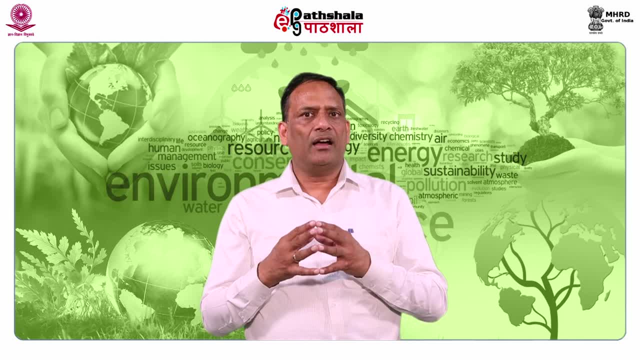 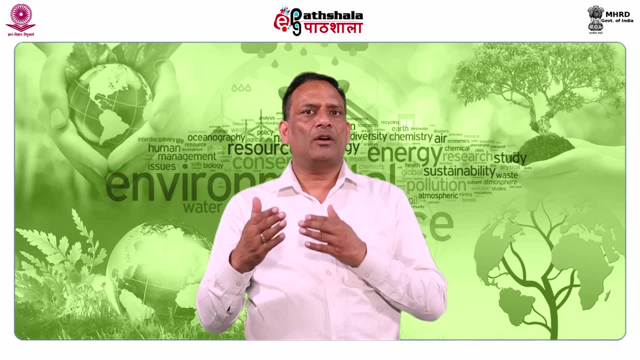 To begin with, fossils provides an idea about the age of the petroleum source rock. Secondly, they also provide vital information. The fossil is not an easy topic for our time, So they provide more information. It is as simple as a lamp. 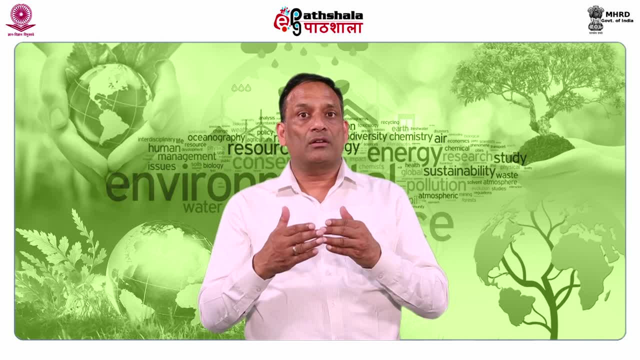 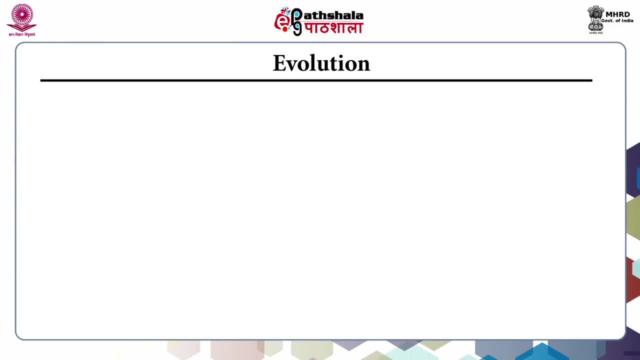 It provides some vital information about the temperature and pressure condition, which are crucial for the formation of coal and petroleum. You can see that the paleontology of the world is having important application in the process of evolution. With the help of paleontology, we can find out information about the evolution process. 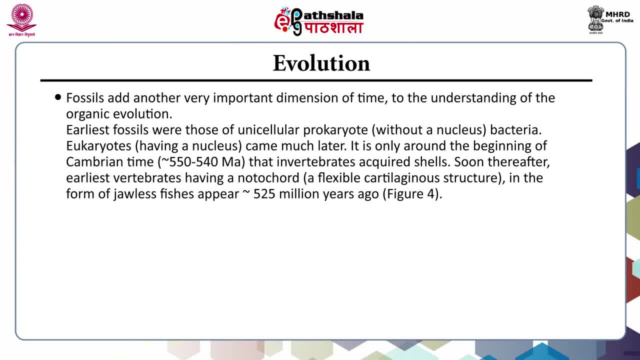 Fossils add very important dimension of time to the understanding of the organic evolution. The earliest fossils were alive in earth. They have evolved for many centuries and their evolution has been an example of that. In fact, they are known for years. 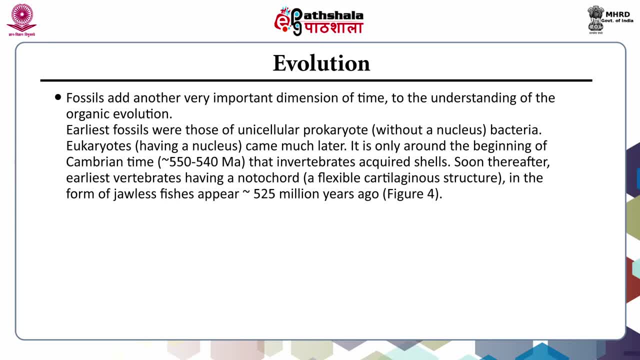 Fossils are the most important natural products. They lead to the evolution of matter. Fossils are the most important natural products. In fact they are the most important natural products. earliest fossil were those of unicellular prokaryotes. You know, prokaryotes are those. 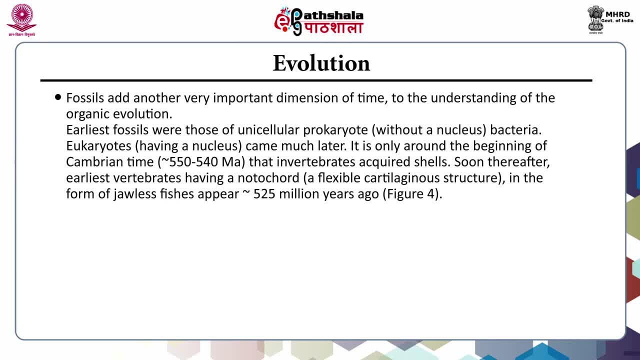 which are not having a nucleus. So the early fossils were those of unicellular prokaryote bacteria. Eukaryotes are those which are having nucleus- came much later. It is only around the beginning of Cambrian time, that is, 550 to 540 million year ago, that invertebrates 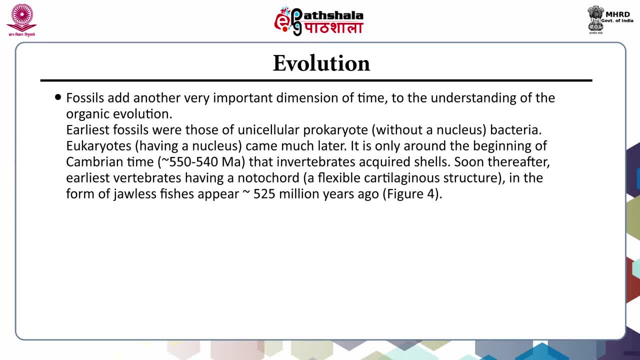 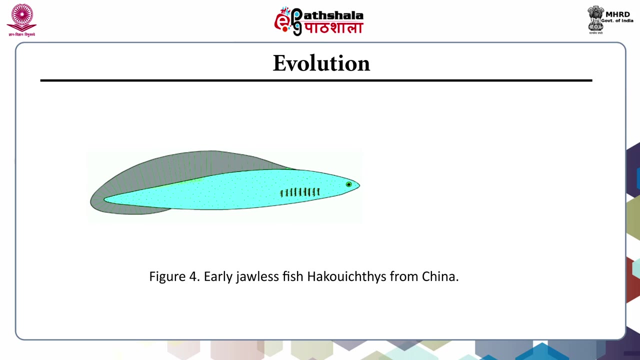 acquired shells Soon thereafter, earliest vertebrates having a notochord, that is, a flexible cartilagious structure in the form of jawless fishes, which appeared approximately 525 million year ago. Here this picture: it is showing the fossil of a early fish, and this fossil is from China. 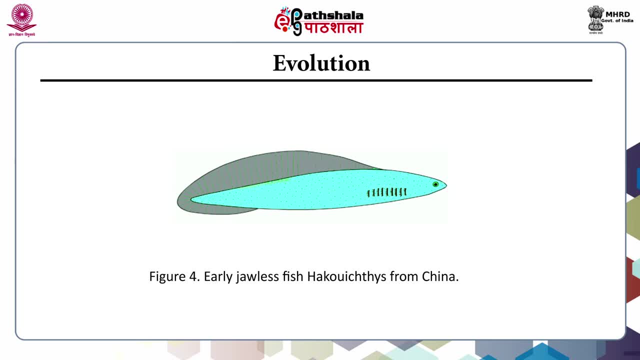 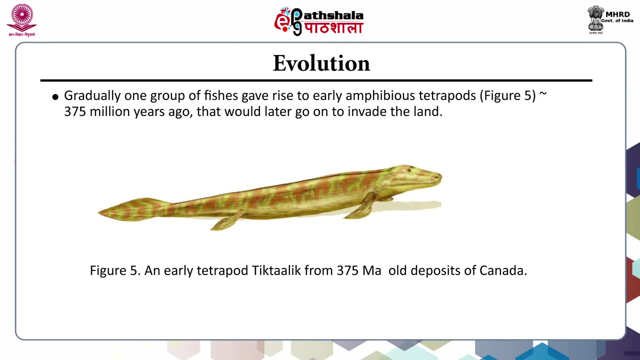 A group of fishes gave rise to the early amphibious tetrapods approximately 375 million year ago that would later go on to invade the land. This figure shows the image of an early tetrapod that existed about 355 million year ago and has been found in the deposits of Canada. 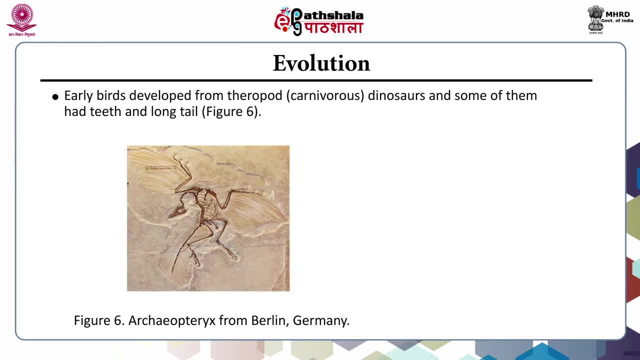 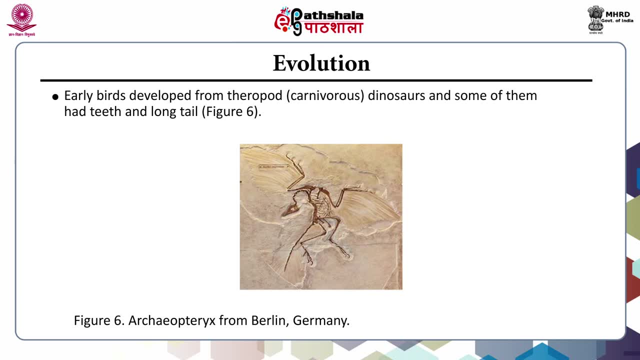 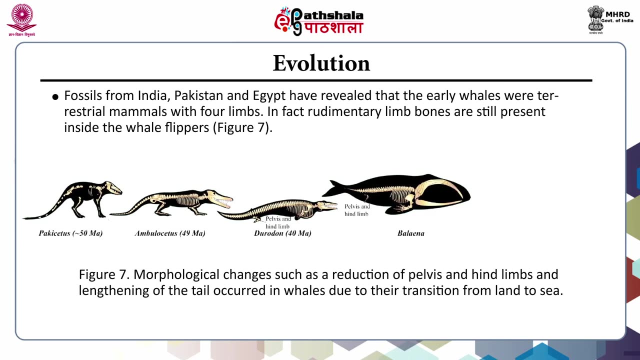 Doouuu opaque region, fungal metropper and ana lithopchaeological digimon. After this, the entire cultures, coasts of the Vlogs were destroyed Due to pelvic erosion. the inshhoret news about this specific prepared successor was: 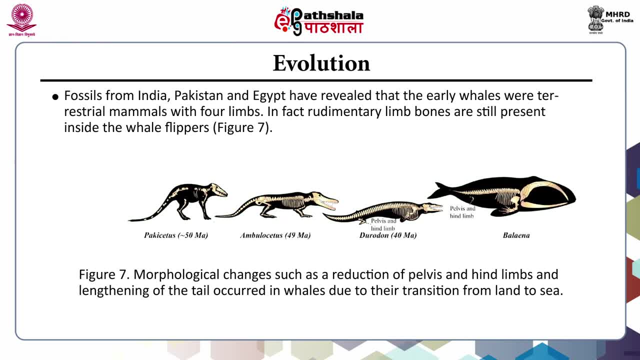 awakened by a species of droünde continent, reported by the University of place Lethe E e番. 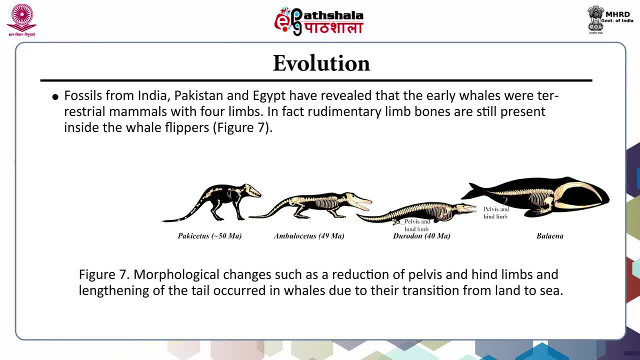 still present inside the whale flippers. So this- all information regarding the evolution of species- can be collected or can be obtained through the fossils. If you look on this figure, this figure shows the morphological changes, such as reduction of pelvic and hind limbs. 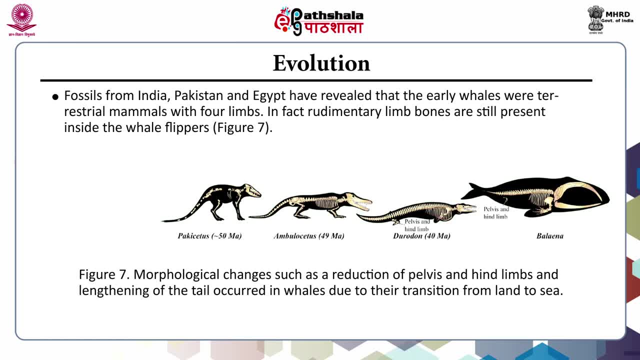 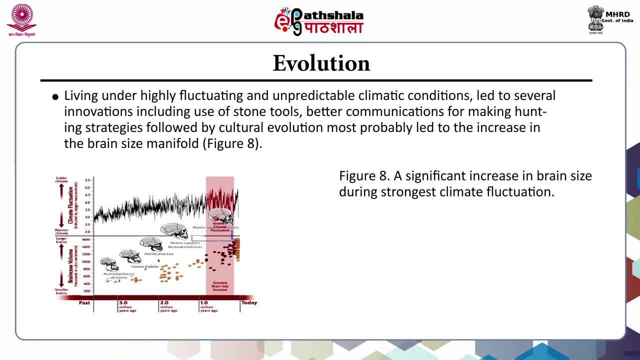 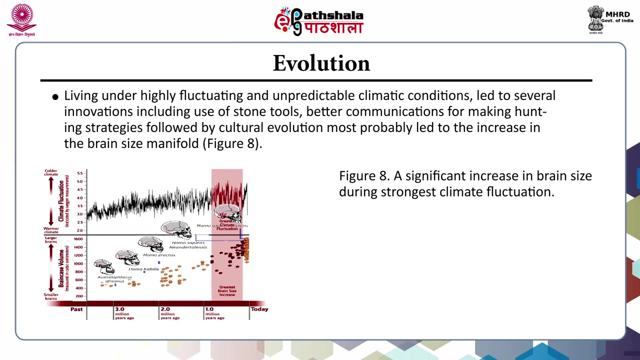 and lengthening of tail that occurred in whales due to their transition from land to sea. Now, this is a very interesting figure. Living under highly fluctuating and unpredictable climatic condition led to several innovations, including use of stone tools, better communication for making hunted, hunting strategies, followed by cultural evolution. 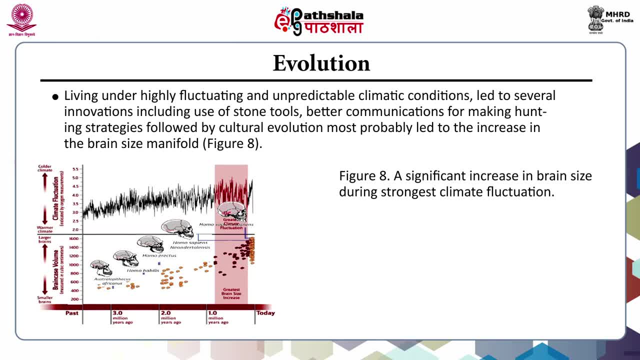 Most probably led to the increased in the brain size manifold. Let you have a look on this figure. In the upper part of this figure, climate fluctuations are shown and in the lower part of this figure, changes in the brain size are shown and this picture climately correlate the. 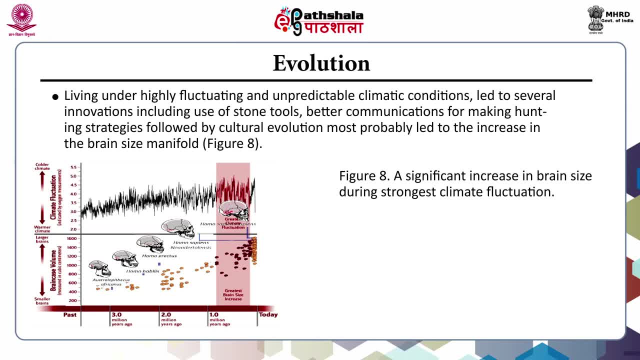 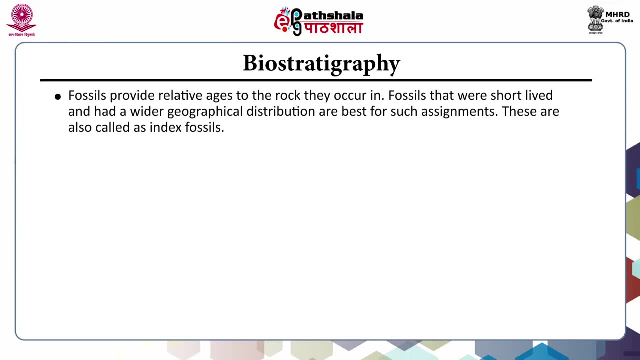 size of the brain with the climate change and you will find that there was a significant increase in the brain during the climate change, So this is a very interesting figure. This is a very interesting illustration showing the strongest climate fluctuation. Fossils have very important application in biostratigraphy. Fossils provide relative 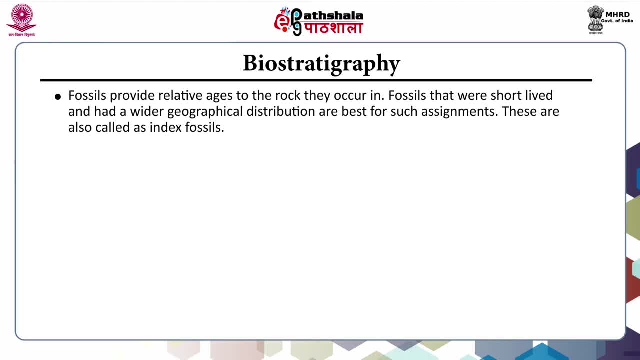 edges to the rock they occur in. Fossils that were short lived and had a wider geographical distribution are best for such assignment. These are also called as index fossils. The occurrence of different fossils together also helps, providing relief. So this figure can. 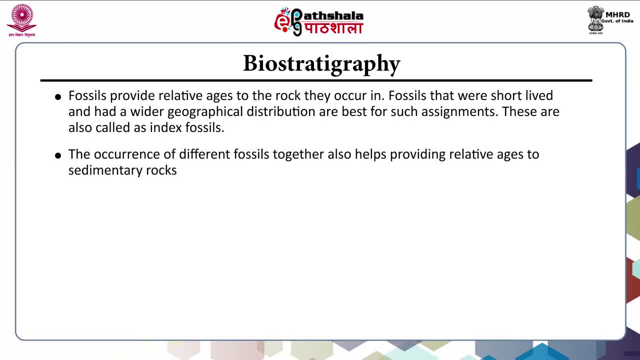 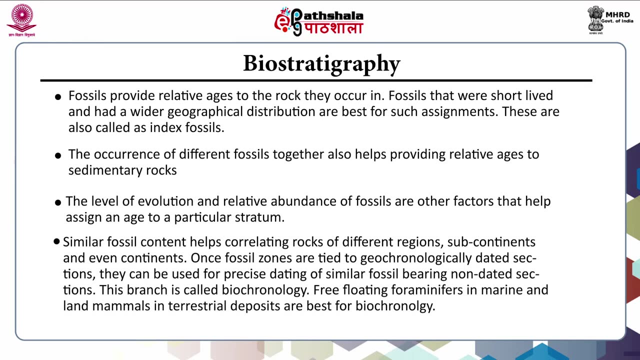 relative ages to sedimentary rocks. The level of evolution and relative abundance of fossils are other factors that help assign an age to a particular stratum. Similar fossil content helps correlating rocks of different regions, subcontinents and even continents. Because fossil zones are tied to geochronologically dated sections, they can be used for precise 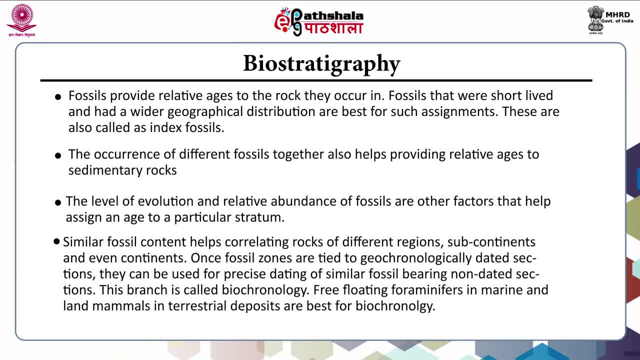 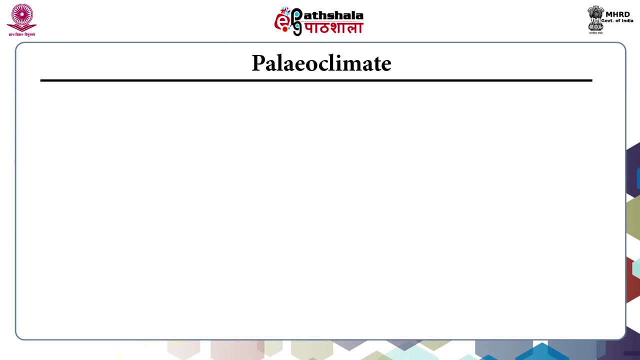 dating of similar fossil bearing non-dated sections. This branch of paleontology is called as biochronology. Free floating from any furs in marine and land, and land mammals in terrestrial deposits are best for biochronology. Now the application of paleontology in paleoclimate past organism sensitive to climate change. 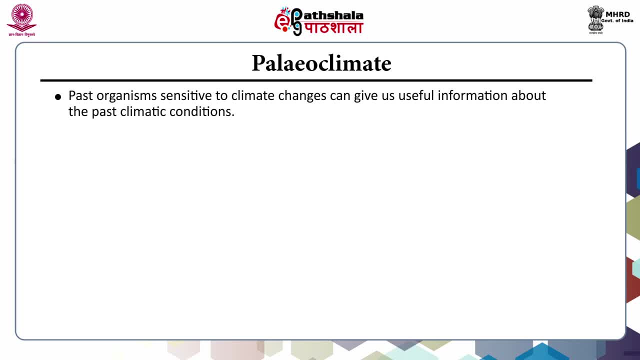 can give us useful information about the past climatic condition. Let me take an example. If one is interested to find fossils of crocodile in 1 million year old rock occurring in Antarctica today, It would indicate Antarctica had tropical climate, because crocodiles exist in tropical climate. 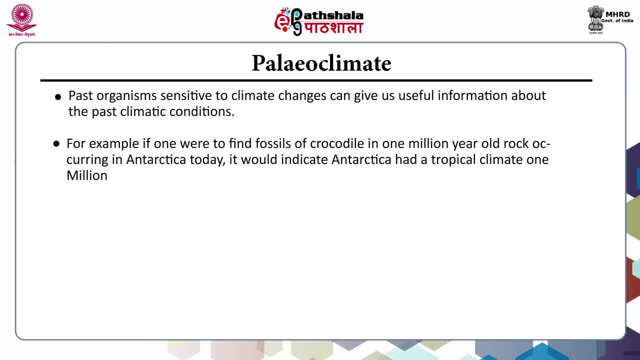 So we can say safely that Antarctica had a tropical climate 1 million year ago. Similarly, life shape is another good indicator of climate. Needle shaped leaves such as those of pine tree: they reflect climate conditions, whereas broader leaf of shawl like that suggest subtropical warmth. 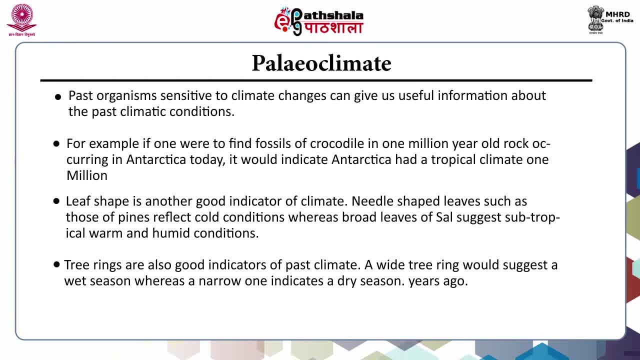 So based upon the type of the leaf, whether it is needle shaped, whether it is broader, we can decide that what kind of climate existed in that area in the past. Similarly, tree rings are also good indicator of past climate. A wide, a wide tree ring would suggest a wet season, whereas a narrow one indicates a dry. 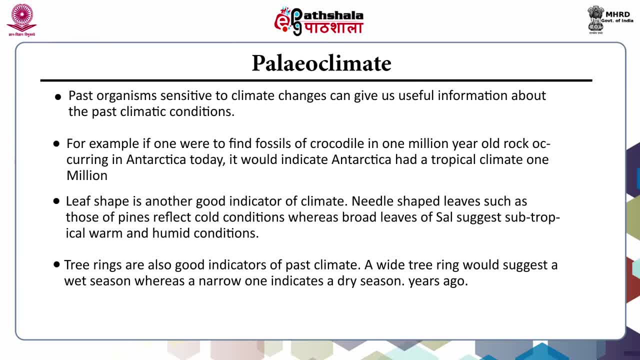 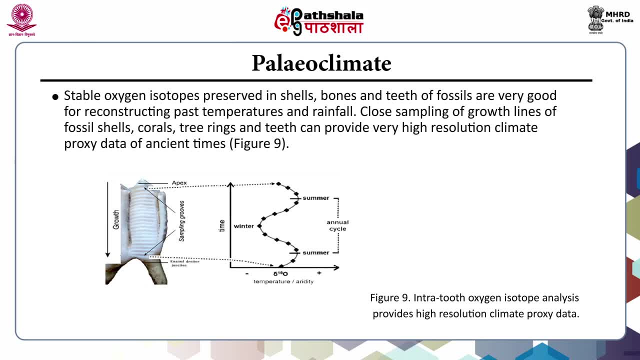 season that existed in that particular area. Stable oxygen isotopes preserved in shells, bones and teeth of fossils are very good for reconstruction, reconstructing past temperatures and rainfall. Cloth sampling of growth lines of fossil cells, corals, tree rings and teeth can provide very. 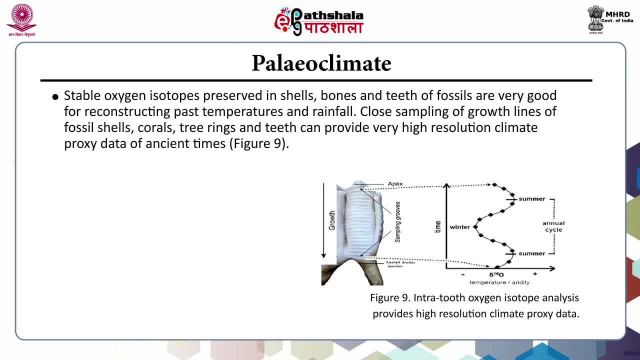 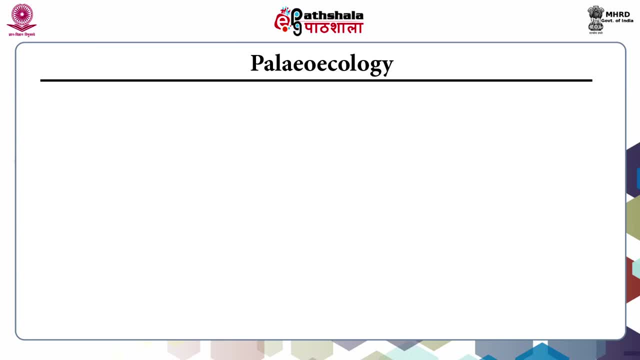 high resolution climate proxy data of azimuth. The next slide. Next slide. So let us look at the application of paleontology in paleoecology. A better understanding of relationship among present day coexisting animals and plants and their environment can help us reconstructing past ecological conditions. 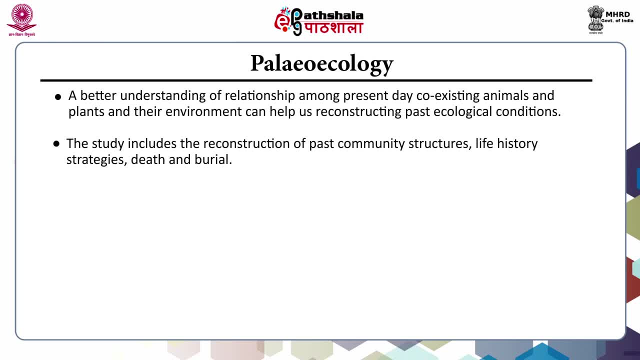 This. this study includes the reconstruction of past community structures, life history, strategies, Death and burial burial of the animals overall. such data, added with physical parameters, help reconstructing paleoenvironmental condition. Past ecological conditions can be built on the principle of actualism, that is, by assuming 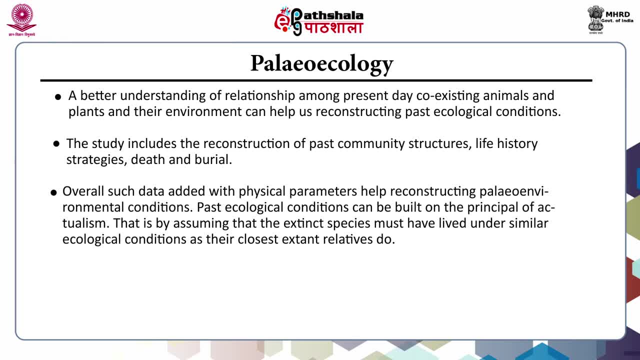 that the extinct species must have lived under similar ecological conditions as their closest extinct relative date. Other procedures involve the analysis of functional morphology. Longer legs are meant for running. if we find several fossil mammal species with long legs at one particular time, it would indicate the presence of an open habitat in that area.